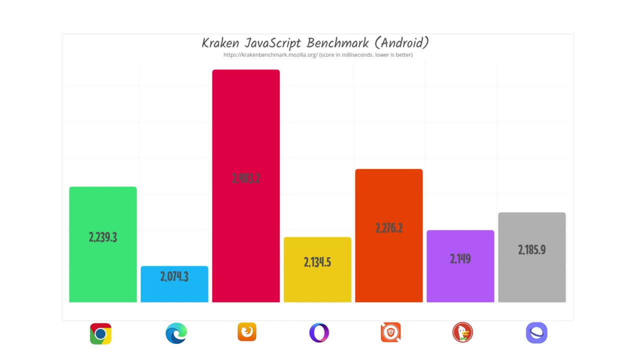 is actually the better because this is measured in the responsiveness, in milliseconds, And we can see that Firefox did not do very well whatsoever, coming in at 2,483.. But in first place, to my surprise, was Microsoft Edge, and that is followed up very close by both Opera, Touch and DuckDuckGo. 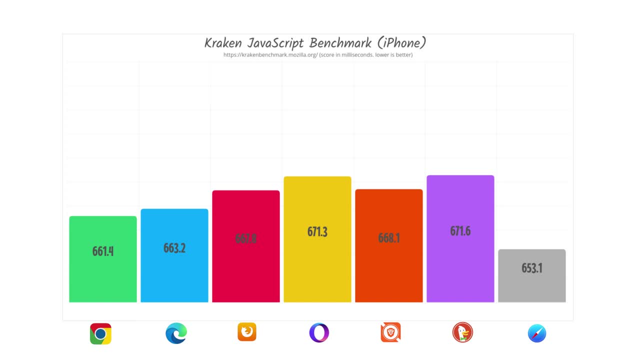 Pulling up the results for the iPhone, we see a much closer situation. So we have a set of scores here, with their default browser, Safari, coming in with the best score on this old school JavaScript test. And the next JavaScript benchmark we ran was Jetstream 2. This 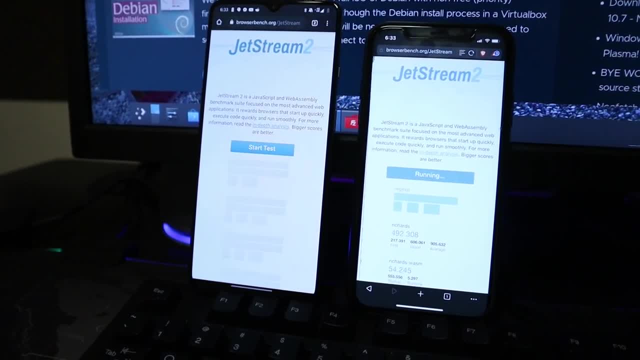 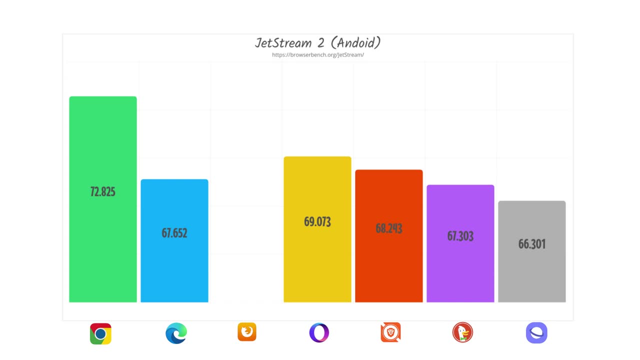 one also does web assembly tests with a focus on advanced web applications. Now these Jetstream 2 scores give us a little bit different result, with Google Chrome coming into the lead. In this case, the scores at the highest are better Followed up by Opera Touch by just three points at a score of 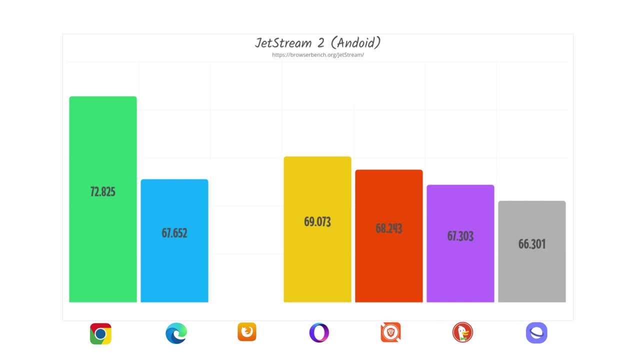 69.. And I will note, in this test, Firefox was not able to run at all, so that is why it does not have a score for this benchmark. And I will also note that this is fairly zoomed in when you are looking at this graph, because there's only really a. 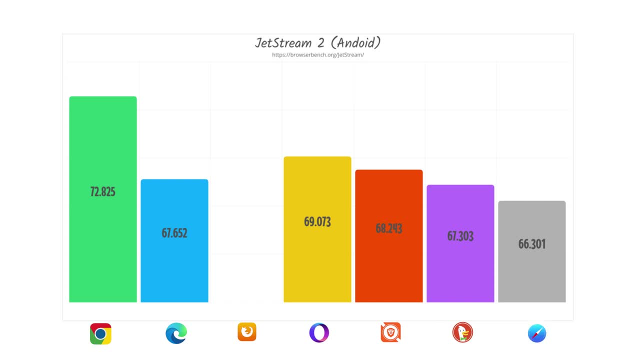 difference of six points between the lowest, which was actually the Samsung browser, and Chrome, which came in at 72.. Now, pulling up the results for the iPhone, we can see that Google Chrome does still have the number one spot at 142, but this time Firefox was. 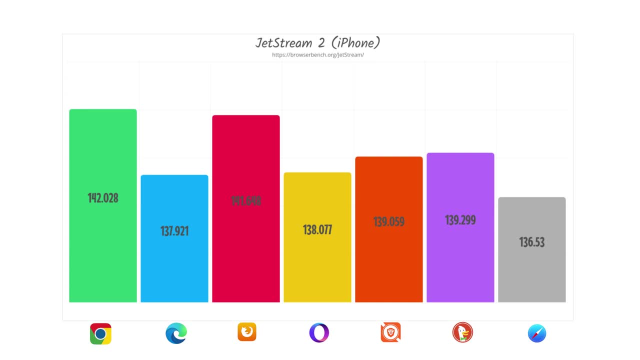 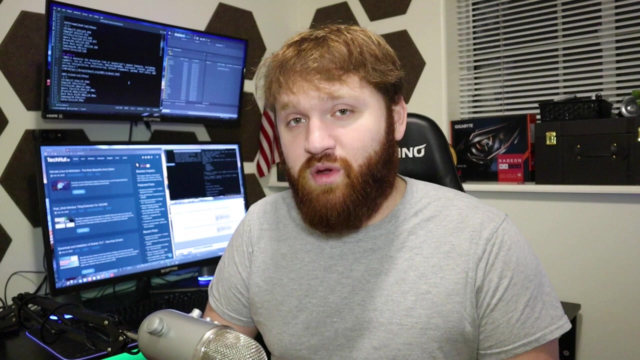 actually able to run and because of that, it came in in the second place spot, falling behind Chrome by less than one point. All the other web browsers are fairly neck to neck, but we do see that Safari did come in last place in this test. Finally, we have ARES-6, which is a JavaScript benchmark that focuses on some of the newer features of JavaScript, such as: 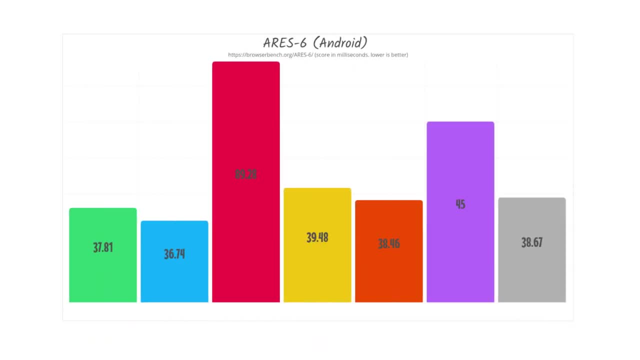 arrows, proxies and things like that. Now for this benchmark. this is another case of the lower the score the better, And with that we can see that the Firefox did horrible compared to some of the other ones, at over double the time it took to execute some of the newer JavaScript features. 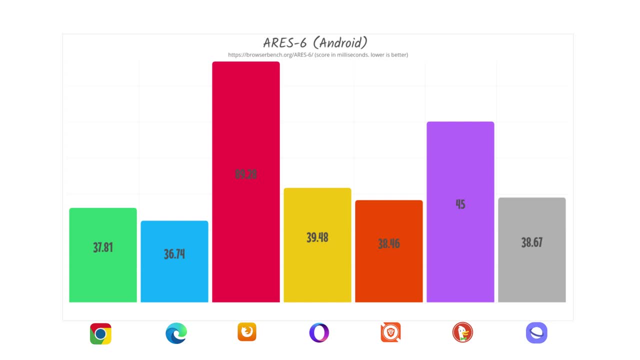 Taking a look at DuckDuckGo, it scored a 45, but that is still the second worst, with all the other ones scoring roughly 36 to right about 40. And in this test, Microsoft Edge actually came in the lead, followed up closely by Google Chrome. 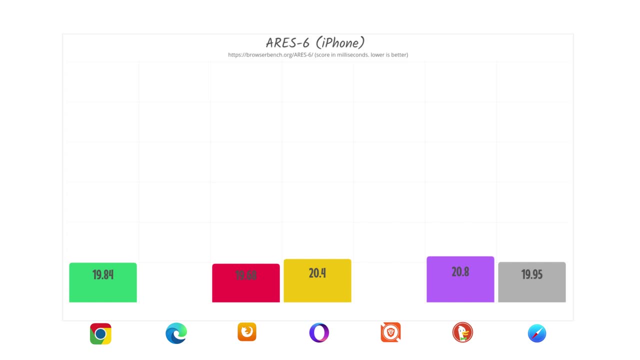 Now taking a look at the results on the iPhone, you can see these tests ran a lot quicker across the board, But I did have errors running this on both Edge and the Brave Web Browser And you can see that all the tests that did run were so neck and neck we could basically call this a tie. 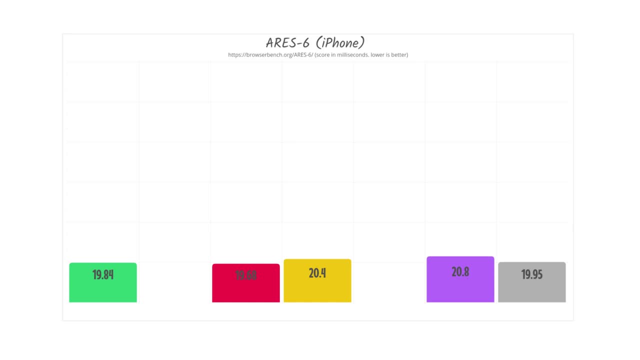 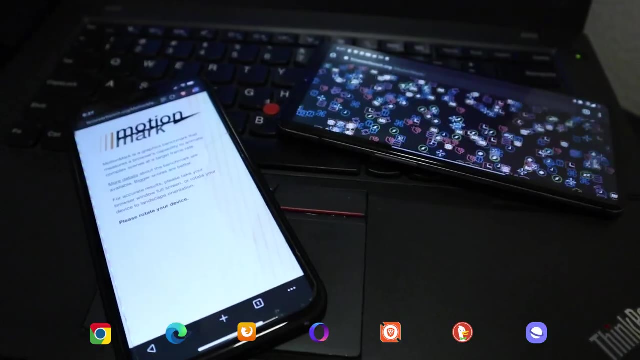 But just for the sake of declaring a winner, Firefox did slightly score the best in this, And now we ran a graphical benchmark called MotionMark, which actually renders out various scenes To help measure your systems performance when it comes to rendering the scenes out at certain target frame rates. 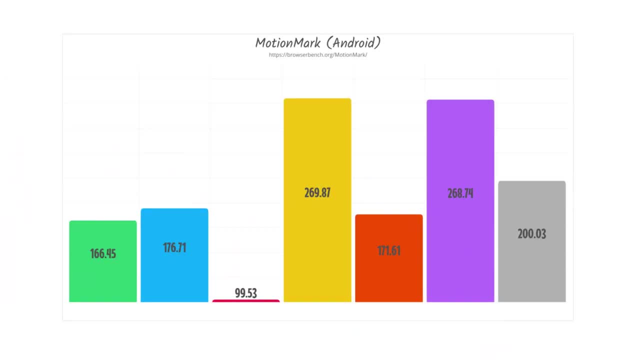 And now, taking a look at this graphical benchmark benchmark on the Android, we do see some rather interesting results, with both Opera Touch and DuckDuckGo actually scoring really, really good, coming in at 269 and 268, followed then by the Samsung web browser at 200, and we can see, in this test, Firefox again did not perform very well. coming in at under 100 points. Both Google Chrome and Edge were fairly close, but Edge did have the advantage. Now, on the iPhone, things do tighten up a little bit, but DuckDuckGo did come out with a very impressive result of 841, compared to the average range of 690 to 720 for a majority of 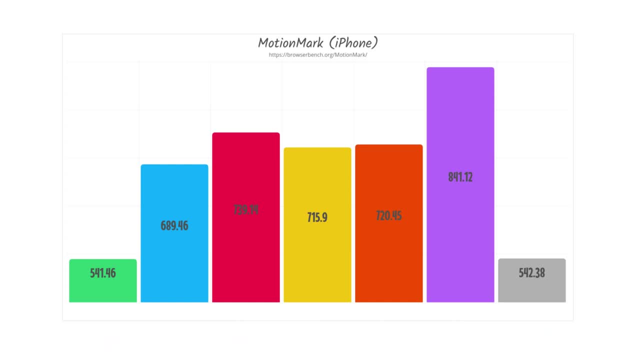 the other tests, but falling behind in this was actually Safari at 542, and scoring last place was Google Chrome at 541.. Now we went ahead and ran a tool called Speed-O-Meter, which just measures the distance between the iPhone and the device. Now we went ahead and ran a tool called Speed-O-Meter. 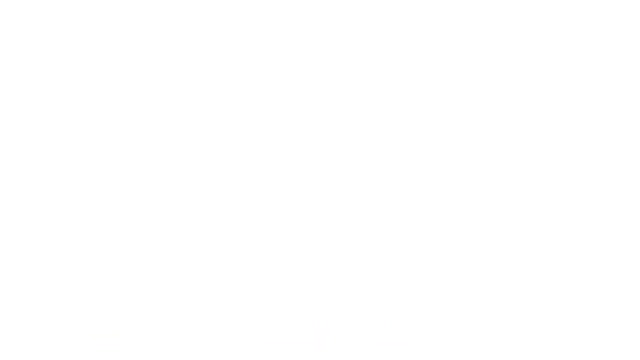 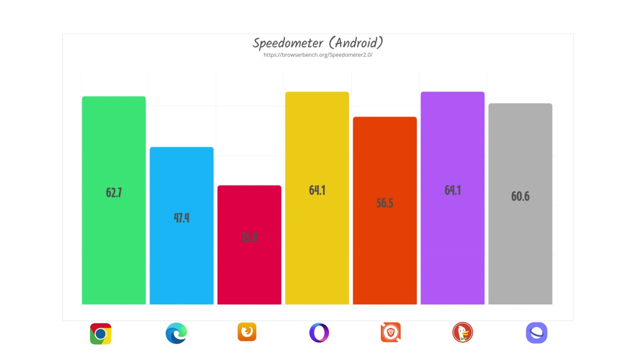 general responsiveness of the web browsers. Now, when it comes to testing the overall responsiveness on the Android, we do have a lot of scores tightening up, but this is another case of Firefox coming in last place at 35, and then we have a tie for first place between Opera Touch. 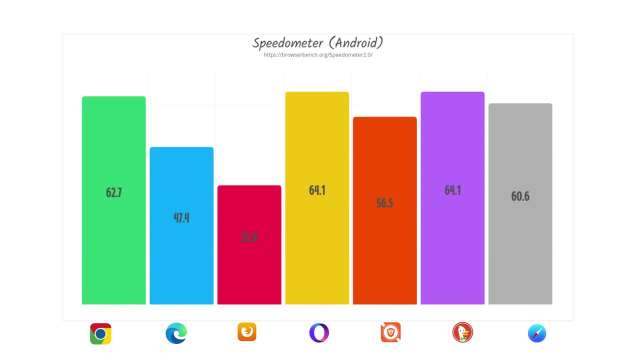 and DuckDuckGo at 64, and then they're followed up by Chrome at 62,, Samsung by 60, and then Microsoft Edge at 47.. Now, looking at the responsiveness of these browsers on the iPhone, we do have a little bit more variation, and the first thing I noticed is on this test. 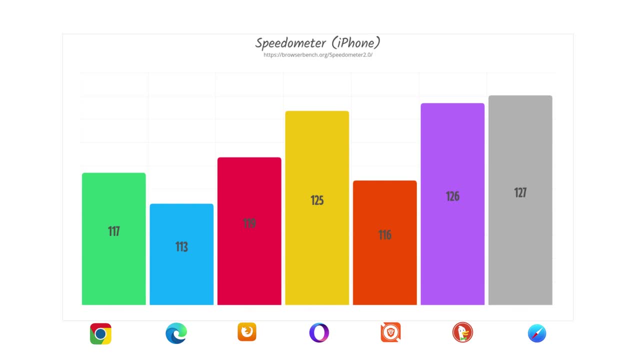 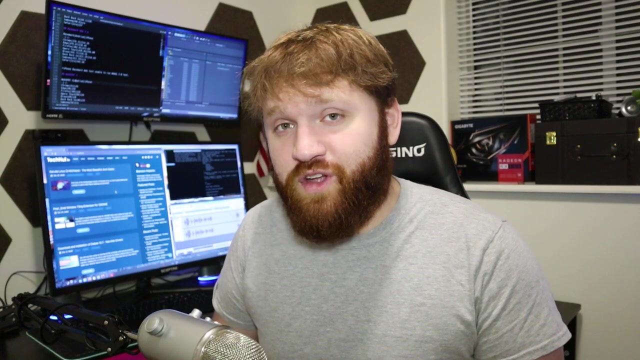 Safari actually came out barely in the lead by one point over DuckDuckGo, followed up by Opera Touch, again barely just by one point. and at least in this test Microsoft Edge did score the lowest, being the least responsive web browser. Now the last two tests we're going to run are larger. 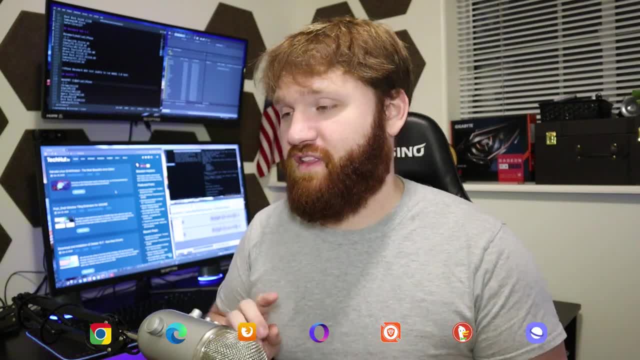 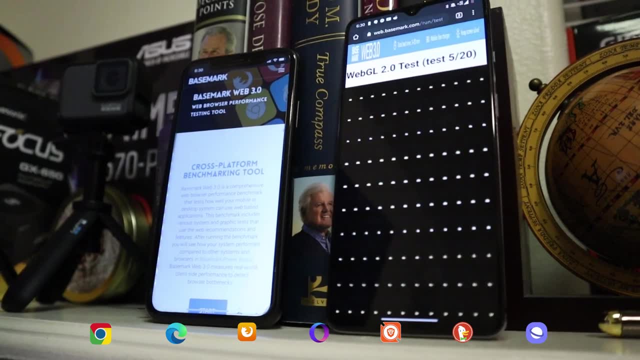 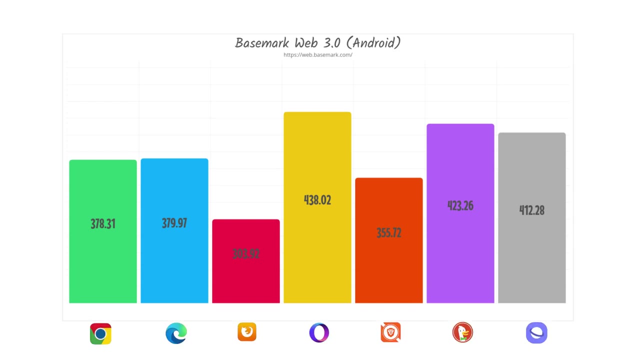 benchmarking suites that do a wide variety of different tests, including the actual system tests, graphical HTML5, and a couple different things, and the very first one is Basemark Web 3.0.. Now, on the Android, taking a look at the results of our first non-specific benchmark score. we have Opera Touch. 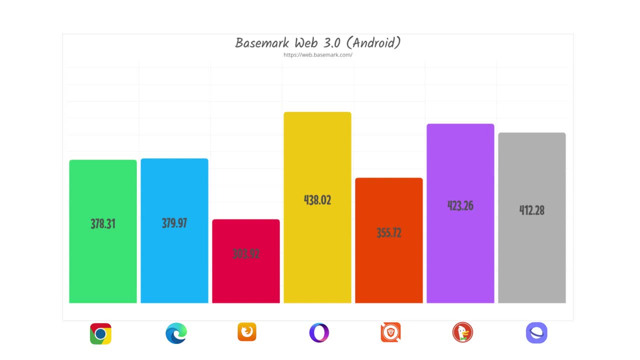 coming in the lead at 438, followed up by DuckDuckGo at 423 and closely behind that is actually the Samsung web browser at 412. and then we look over at Chrome and Microsoft Edge and they're basically a tie with a slight advantage over the other two tests. Now on the Android, taking a look at the 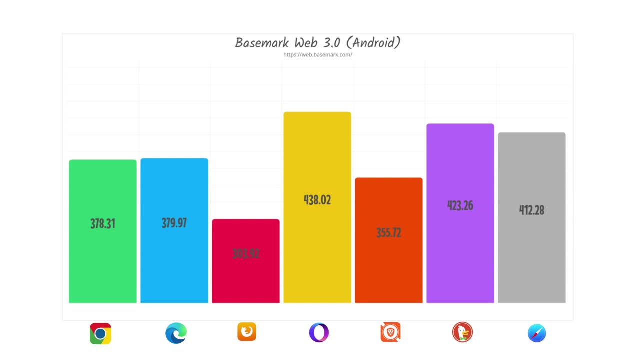 results of our first non-specific benchmark scores. we're going to be able to see that they are relatively similar to Microsoft Edge a little along the way, but the term Microsoft Edge came in there. in this test, Сп종k, Microsoft Edge came in last and then Microsoft Edge came in second. 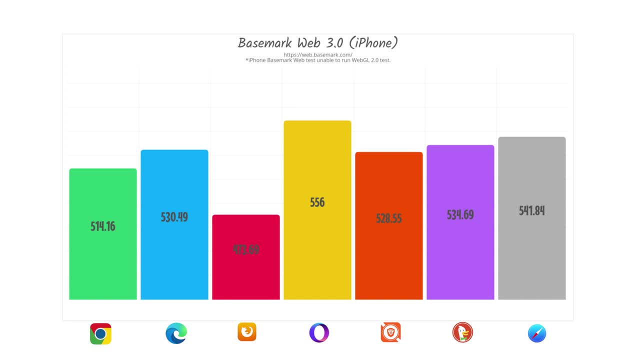 and then, unfortunately, Microsoft Edge at 303.. Now, if we take a look at the iPhone, we do kinda see the same trend, with some differences. I will note that on the actual iPhone, all of these tests failed to run the Web GL 2.0 tests. Being that all of them failed it, we can still use these scores. to compare them with some of the scores. for the latter, I will note that the score we did see in the first one was pretty good, but here we are at the 10% difference and this time it was really a really bad test. We were able to at least get all these scores and score a fair share in the end of. 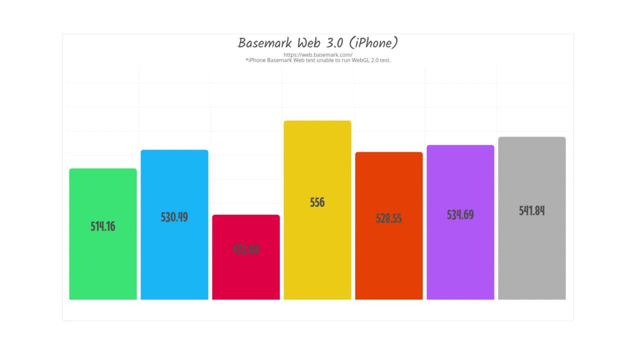 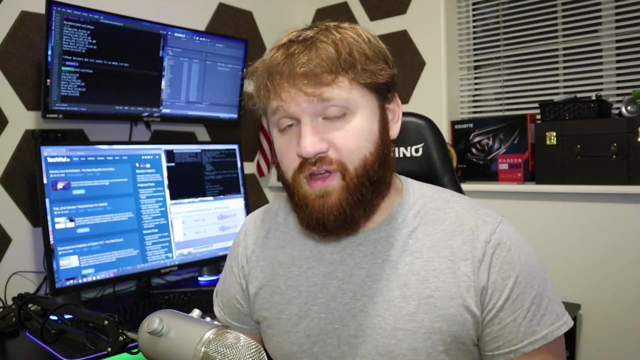 And coming in first place was Opera Touch at $556, followed up by Safari at $541,, and everything else from there was pretty close, but Firefox came in last place at $473.. And now the very last test that we're going to run is WebXPRT3,, and this one's my favorite. 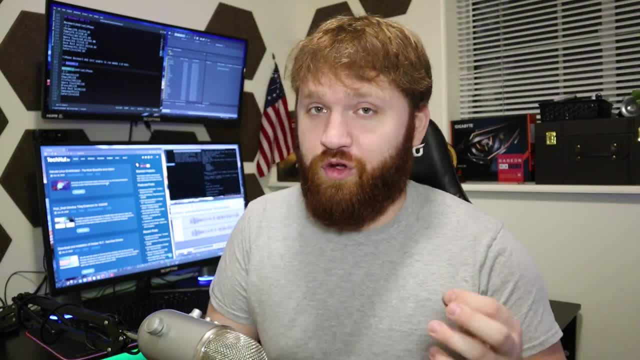 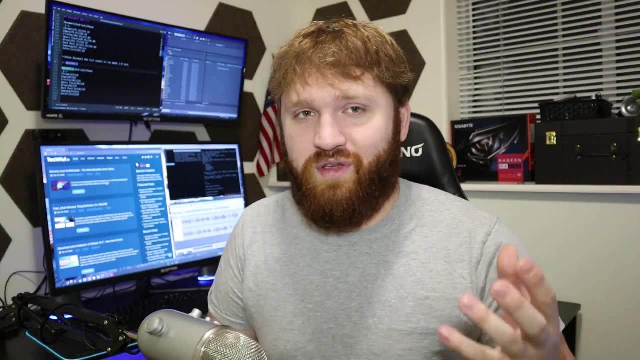 of all the tests because it actually puts the web browsers through real-world situations, including photo enhancements, resizing. it has spreadsheet formulas. it does a lot of different HTML5 and JavaScript things and kind of like WebBaseMark. it's more broad. 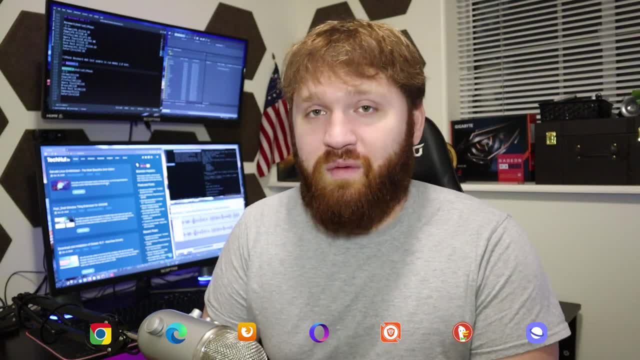 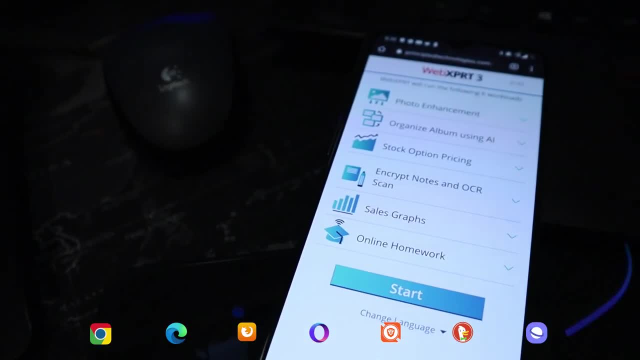 and gives you a generalized score, but this one does do a lot more and it takes a lot longer to run this test And, trust me, running this test on every single one of these web browsers, on both the iPhone and the Android, took quite a while. 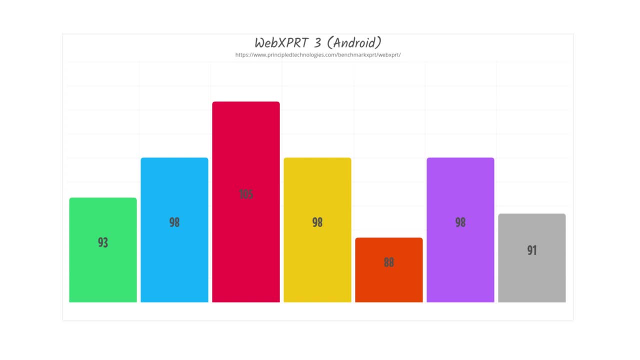 Now, first up in this test we have the Android, and this is actually surprising to me. in these actual use case benchmark testing, Firefox came in the lead, this time at $105, followed up by a three-way tie between Edge, Opera, Touch and DuckDuckGo. 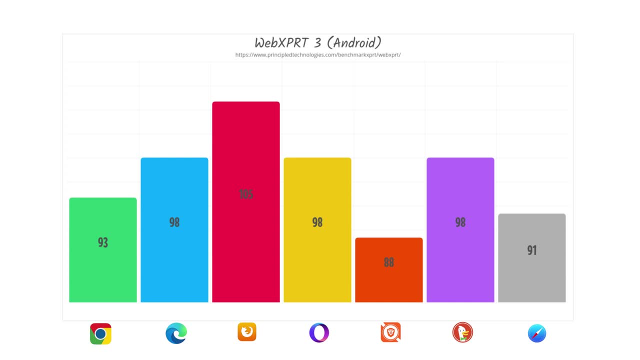 coming in at $98.. Both Chrome and the Samsung browser were pretty close, coming in at $93 and $91, and in this test, the Brave web browser came in last place at $88.. Last but not least, we have the results for the iPhone, and this is one that kind of surprised. 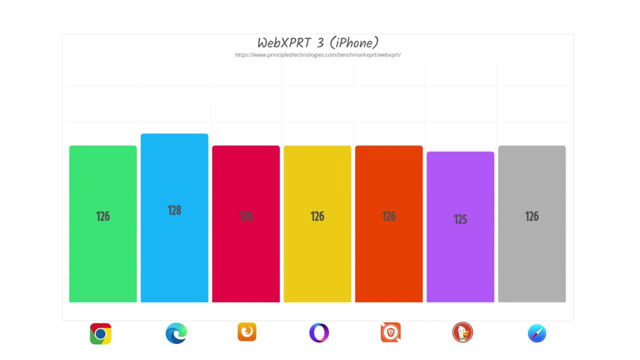 me. Across the board, All of these web browsers seem to be in a tie, with a very slight advantage of Microsoft Edge, and then everybody else, except for the DuckDuckGo web browser came in at $126, and that browser, DuckDuckGo, fell behind just by one point. 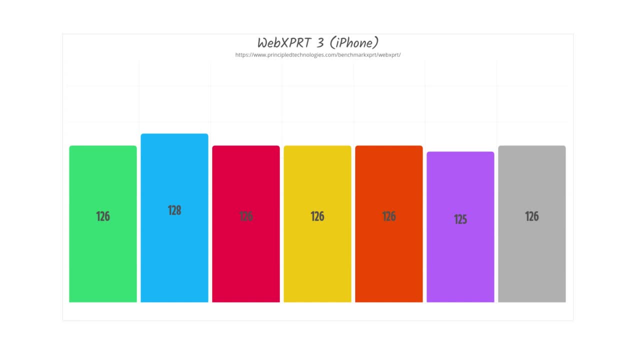 All these results are close enough that you could really just deem this a tie, and I will note on all of these tests I did run this more than once just to make sure there weren't any crazy anomalies. so overall, at least on the iPhone, when you choose your web browser, 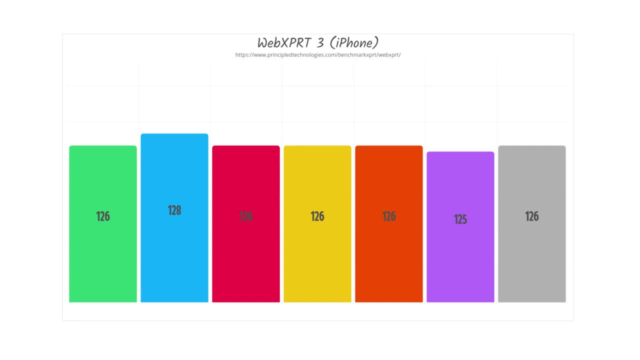 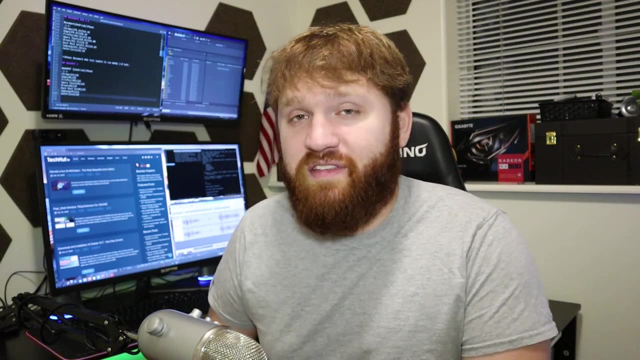 it doesn't matter. It really doesn't matter when it comes to performance, just based on this one benchmark alone. So that about wraps up the scores of the benchmark tests. I know that, personally, I'm going to be taking a look at DuckDuckGo and seeing if I actually 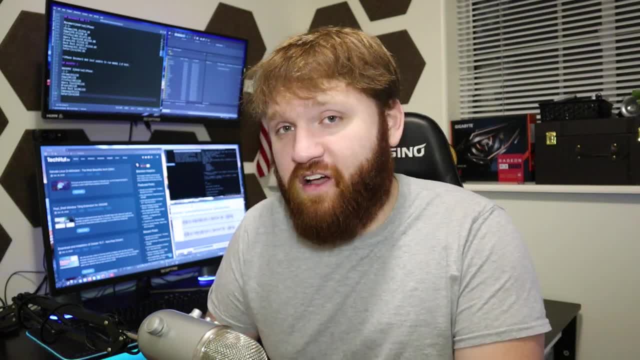 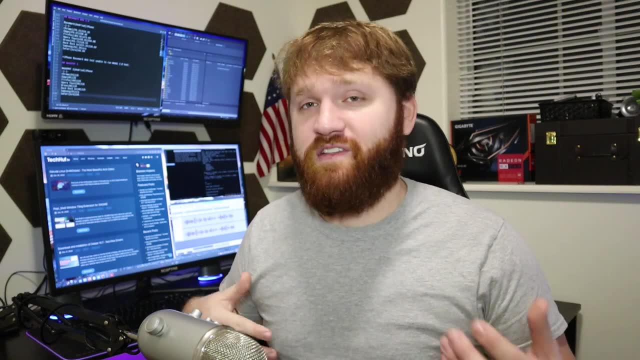 like the web browser. At the moment I've been using the Firefox web browser and personally I like it just because of the UI. I use Firefox on the computer, so I use a lot of the sync functionality and, in reality, 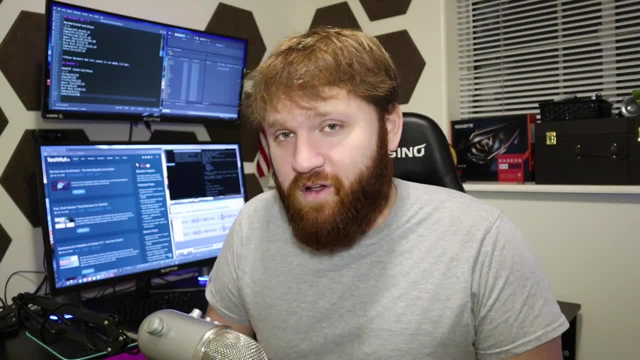 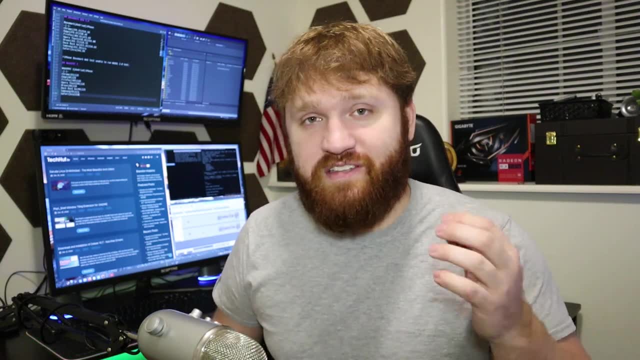 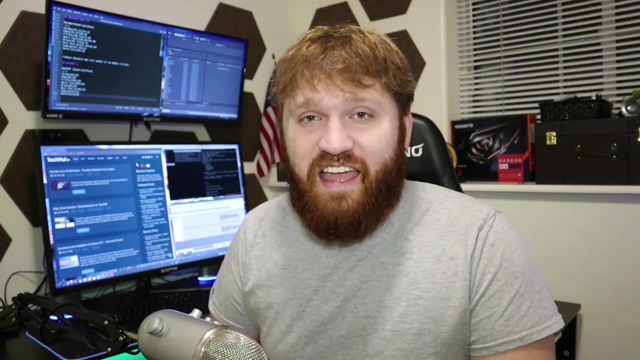 I don't really notice the downfall. I'm just going to take a look at some of the JavaScript scores. and this kind of benchmarking is just one factor in numerous factors to decide what web browser you want to go with. And it is important to note that a lot of these tests we ran are kind of synthetic. 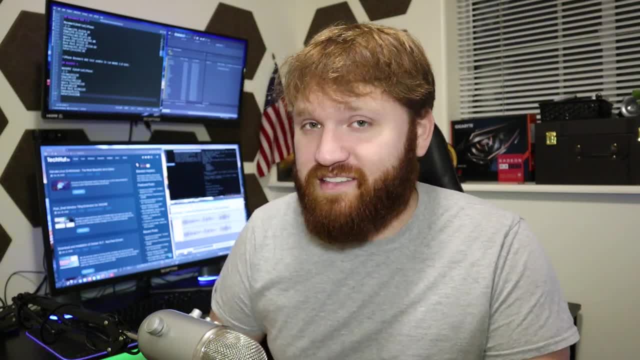 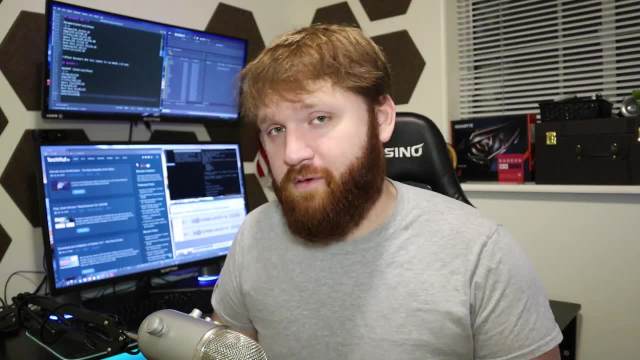 generic tests. If you're going to consider these, I'd almost look more at the last two, unless if you're doing things that are heavy JavaScript-based applications and stuff like that within your web browser on your phone. So my question to you is: did any of these results surprise you? 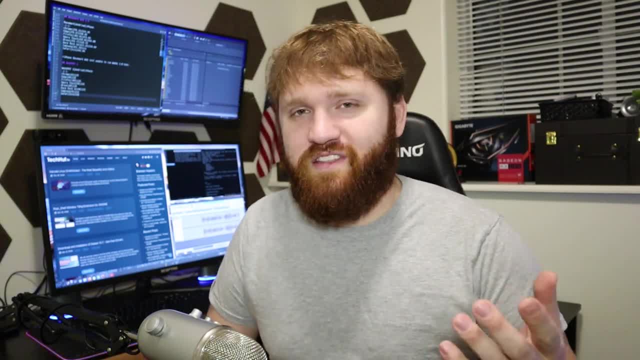 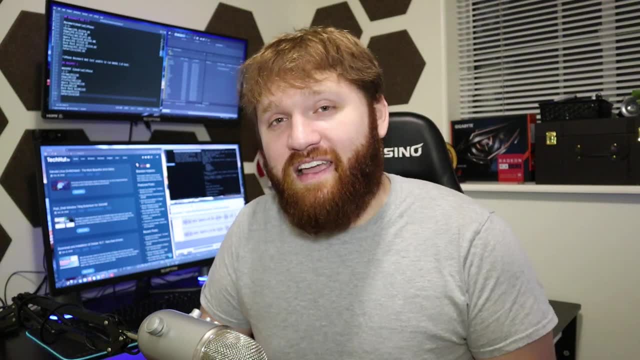 And is there a web browser that you use that wasn't on this list, that you think I should have covered, or anything like that? really, Let's have a discussion down below And if you did like this video, be sure to give it a thumbs up.